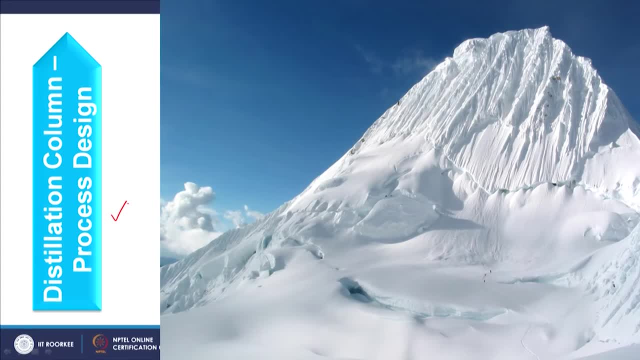 column process design. First of all I am focusing on the process design and then we will proceed for mechanical design. So in the process design we will start with the distillation and the continuous process. It means here I will quickly cover the topic which you have. 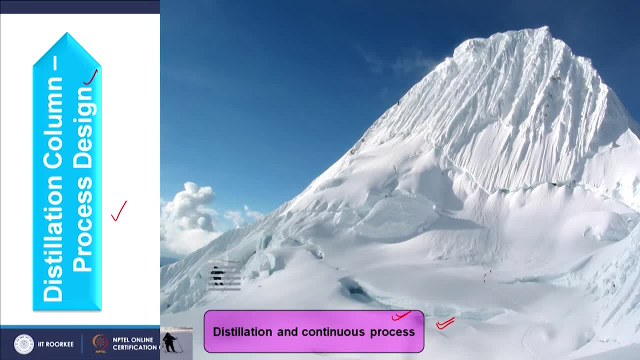 already read. so some revision will be done over here And then we will design the biotech binary system. So this part you also have covered. so we will cover this very quickly and then we can consider multi-component system. So in your B tech second year course you 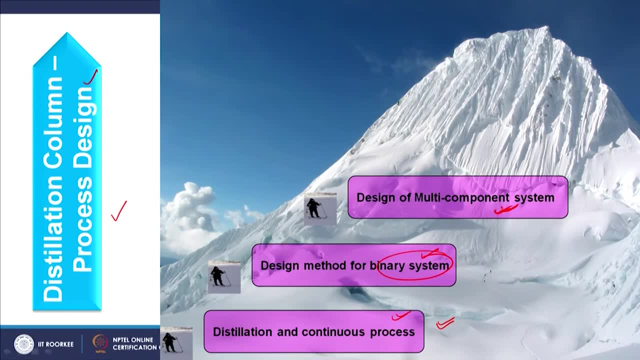 may not have done this, So that will be covered over here right And now, once I am having the multi-component system, we will focus on plate efficiency. efficiency is concerned. some points about that. you already know that we have point efficiency. 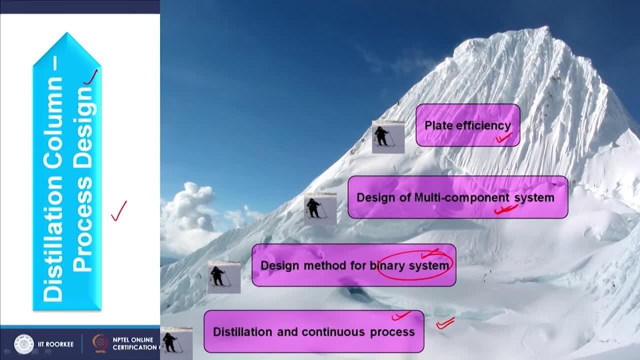 mercury, plate efficiency, etc. but here we are going to discuss plate efficiency in very detailed manner, okay. And finally we can have the topic plate hydraulic design: how to design the plate of a particular distillation column, okay, So in this way the whole process design will be covered. 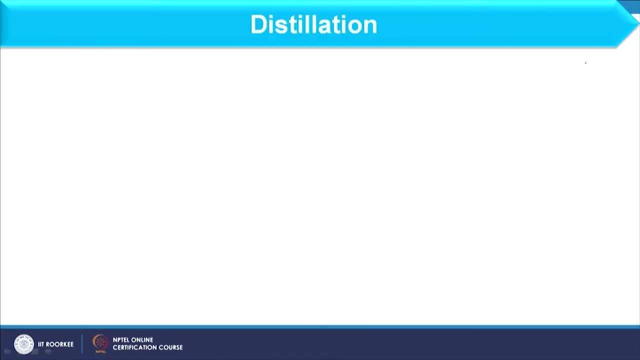 So let us quickly revise the distillation and the continuous process. So, as far as distillation is concerned, it is basically the unit operation in which constituents of the liquid mixture are separated using thermal energy. okay, And that thermal energy we usually provide in the reboiler. 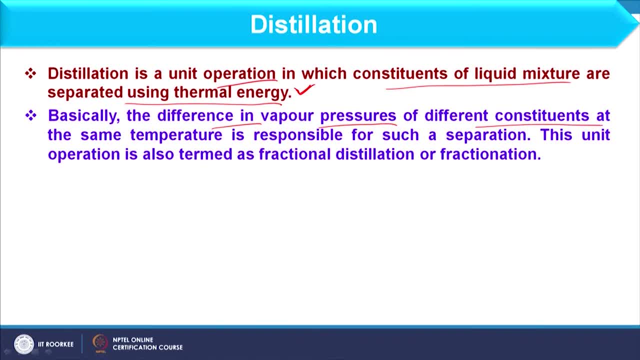 So basically, the difference in vapour pressures of different components, So at the same temperature, is responsible for such separation. This unit operation is also termed as fractional distillation or fractionation right And further, we can have the liquid mixture which is to be separated into its component. 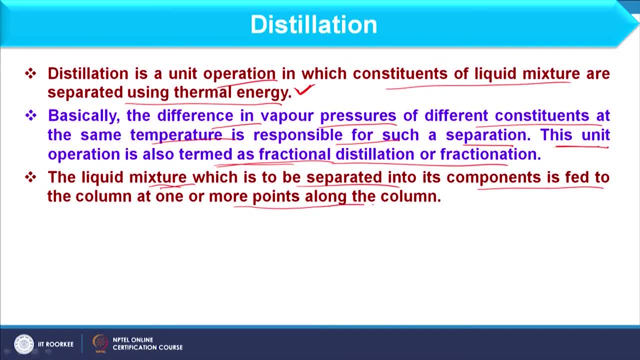 and that should be fed to the column at one or more points along the at one or more points along the column. It means we can have the multiple feed system and distillation column and accordingly we can choose the insertion of the feed right. 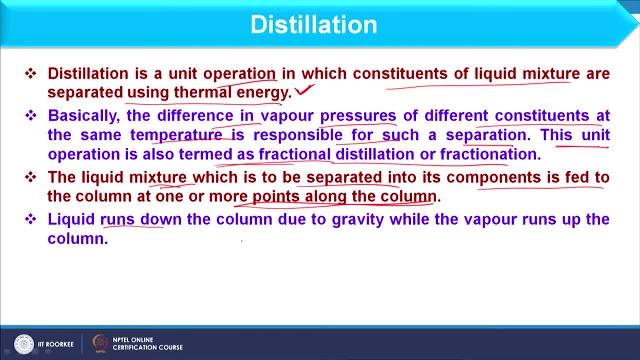 In the distillation column, we observe that liquid usually runs down the column due to gravity, while vapour moves up, which is the natural phenomenon, which is the natural movement of vapour as well as liquid, and vapour is produced by partial vaporization of the liquid. 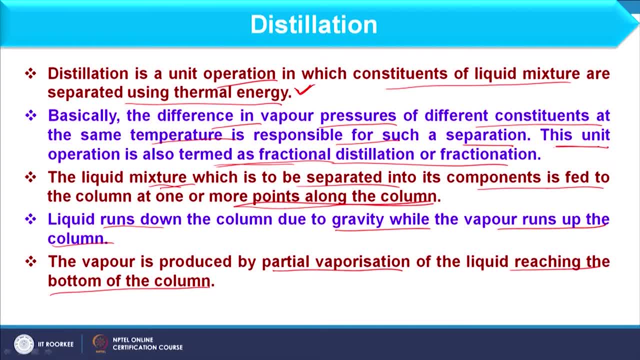 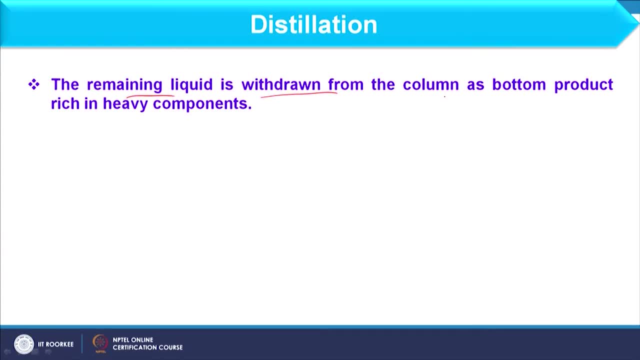 Okay, Okay, liquid reaching the bottom of the column. So here you can consider this. partial vaporization is usually occur in reboilers. okay, So further, the liquid which is remained is withdrawn from the column as bottom product, and that is basically heavy and that contains basically heavy component. okay, 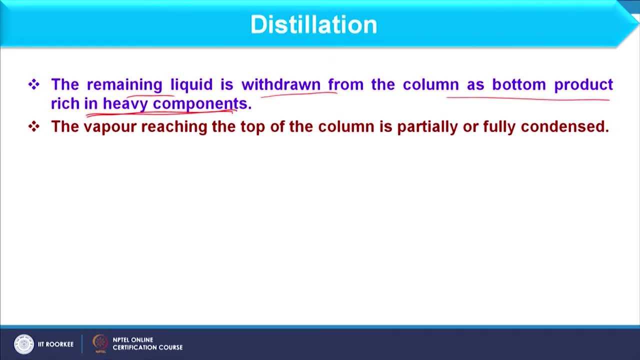 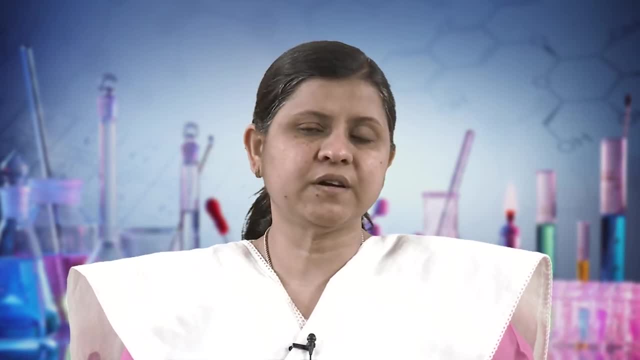 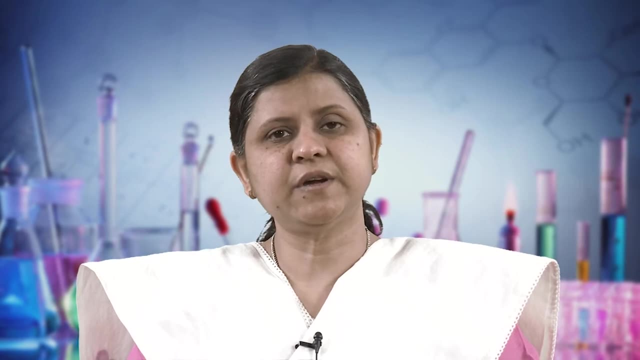 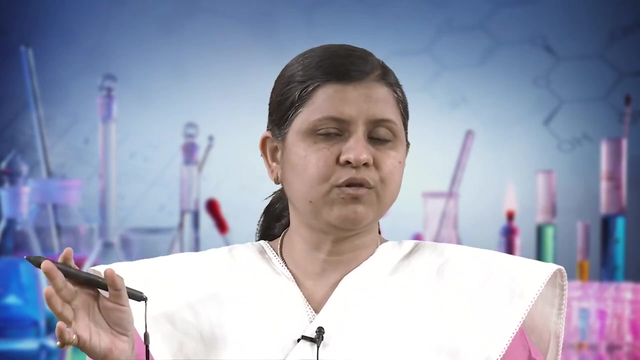 I hope you understand the meaning of light component and heavy component. which is lighter, it means which has more volatility. okay, that will be considered as lighter product or lighter component. fine, Which has lesser volatility, it will be considered as heavy component. okay, and you understand that in distillation column, from top we usually have light component and from bottom we usually 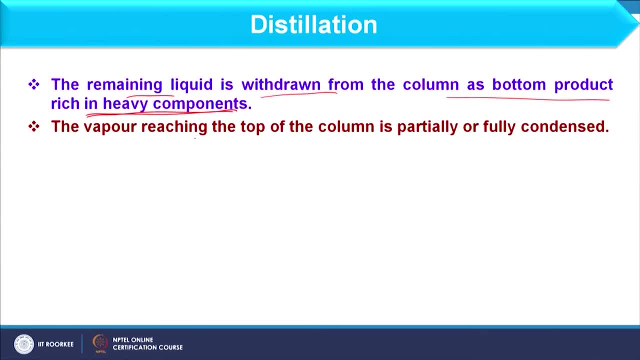 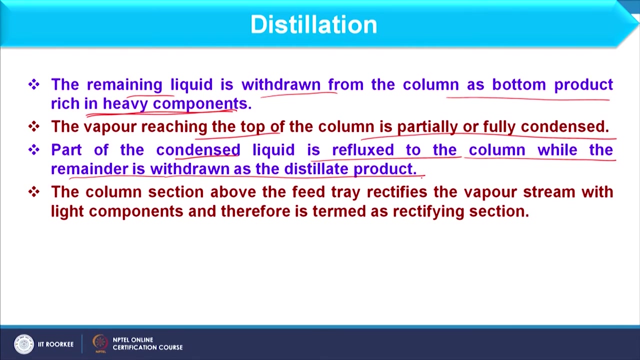 get heavy component. okay. So vapor reaching the top of the column is partially or fully condensed, okay, Part of the condensed liquid is refluxed to the column, while remaining we can withdraw as a distillate product, okay. So all these points you know, but we are quickly covering it and further we have column section. 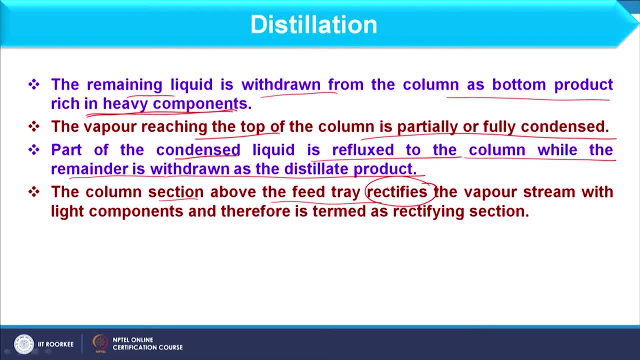 above the feed tray, which we consider as rectifier section or rectifier column. So this is the column section, So this is the column section. So this is the column section, So this is the rectifying section basically. So it rectifies the vapor stream with light components and therefore we consider this. 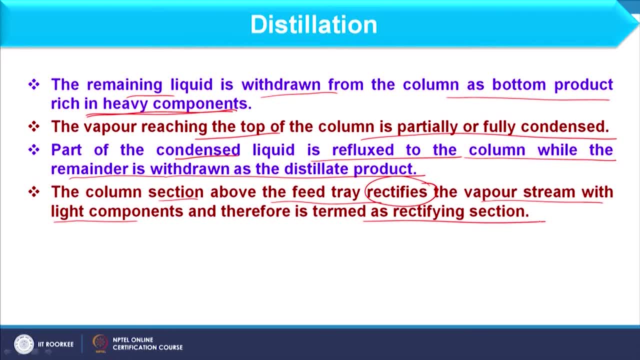 as a rectifying section or rectification. okay. In the similar line, the column section below the feed tray strips heavy component from vapor stream to liquid stream and it is termed as the stripping section. So in this way we basically have lighter product as distillate and heavy product as 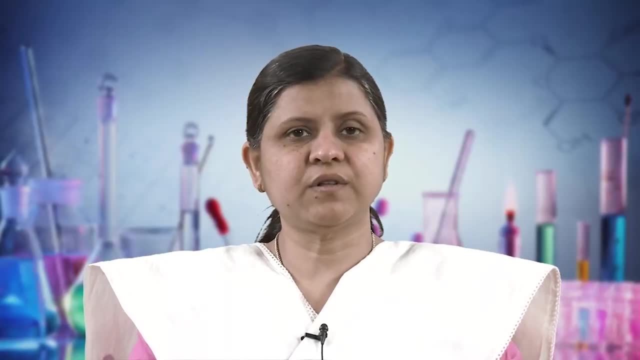 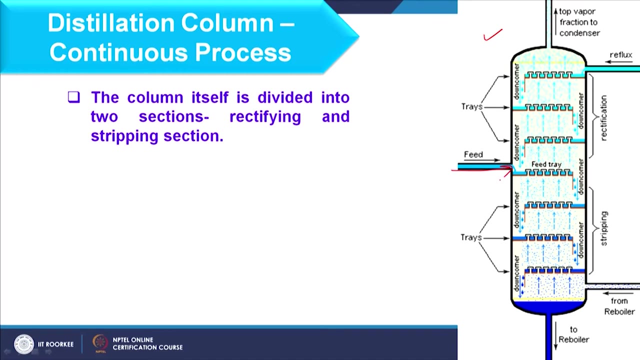 bottom. okay, So let us focus on the continuous process. If you consider this schematic, here we have the feed which is entering into the distillation column, The feed which is entering into the distillation column. The feed which is entering into the distillation column. 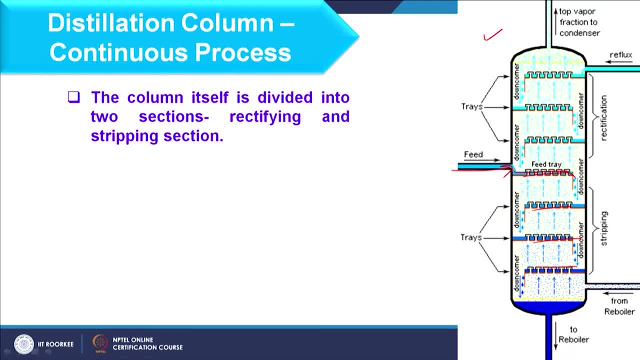 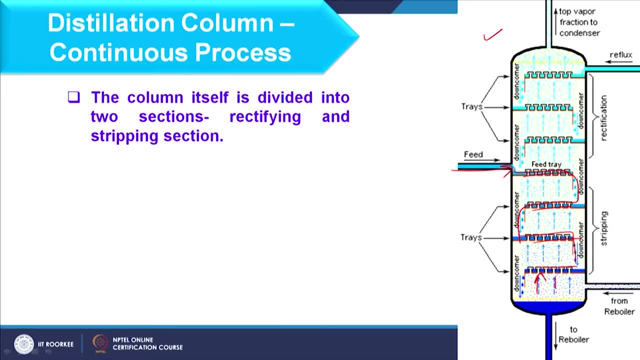 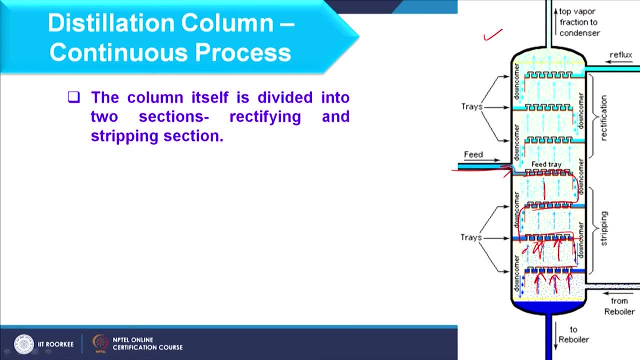 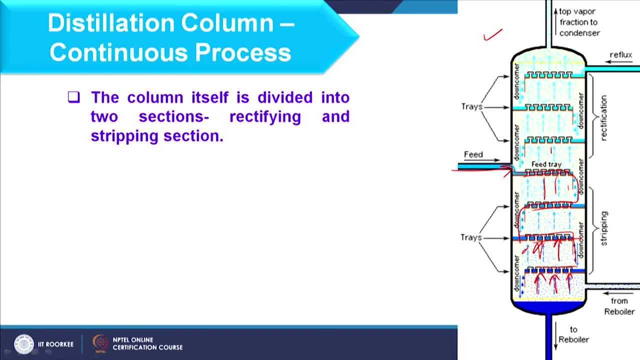 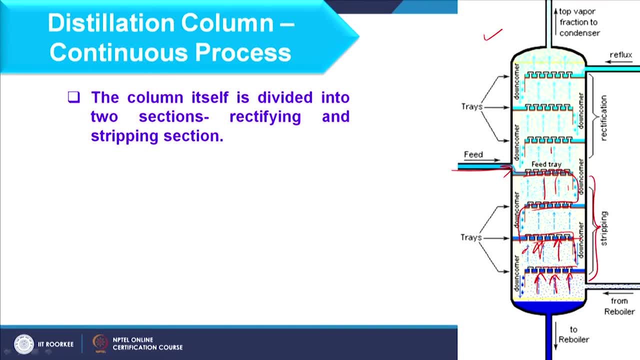 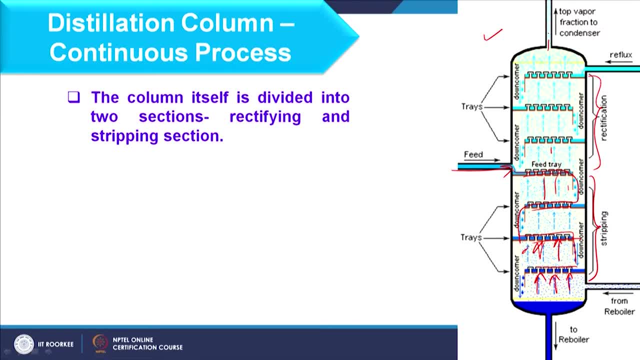 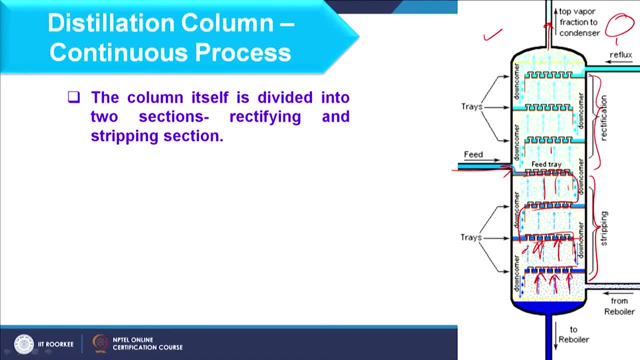 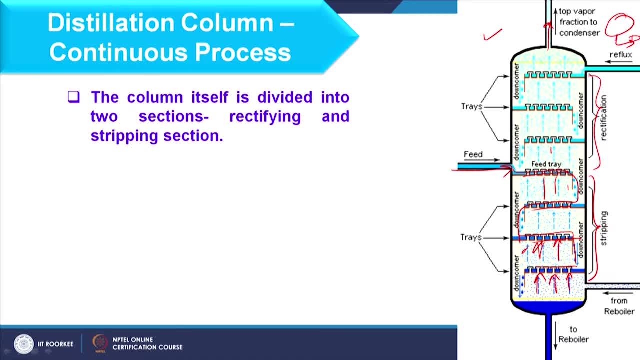 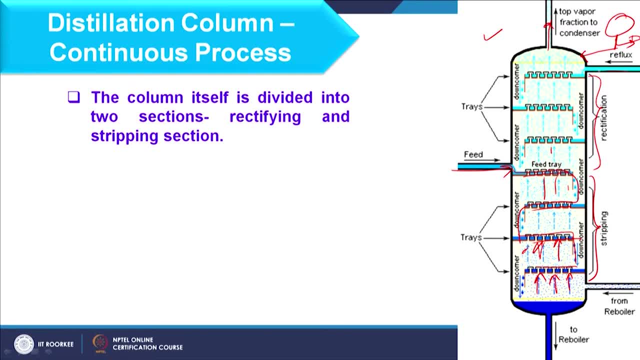 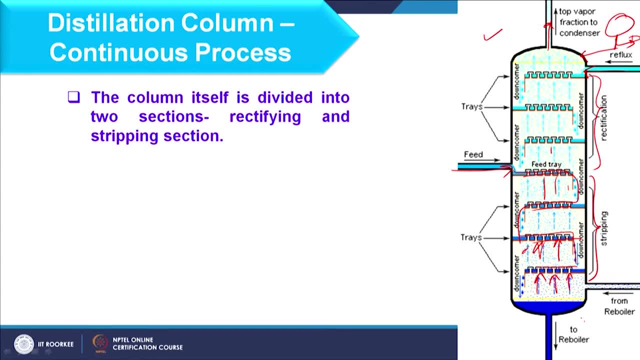 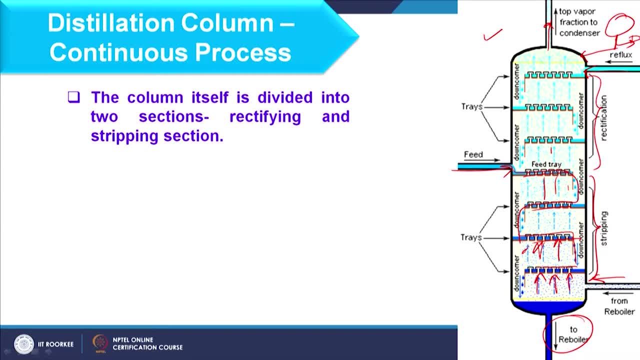 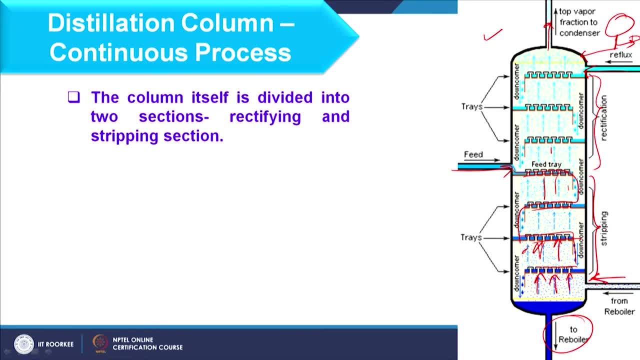 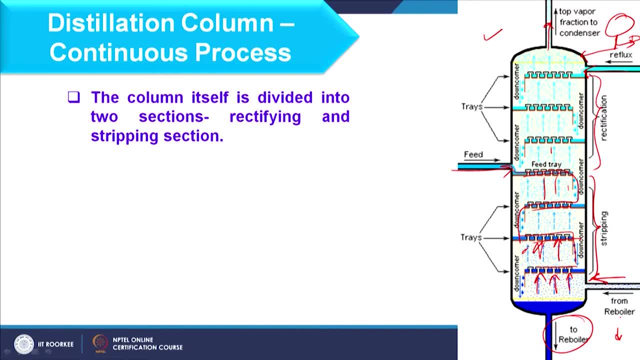 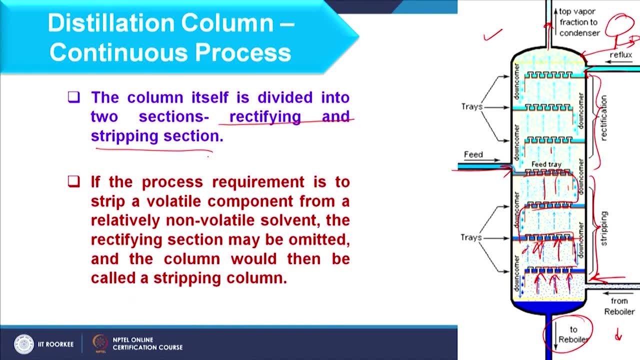 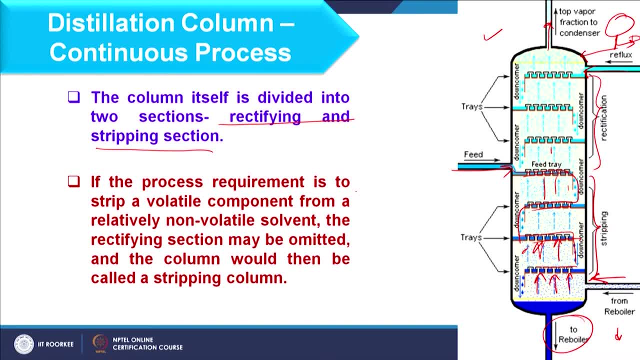 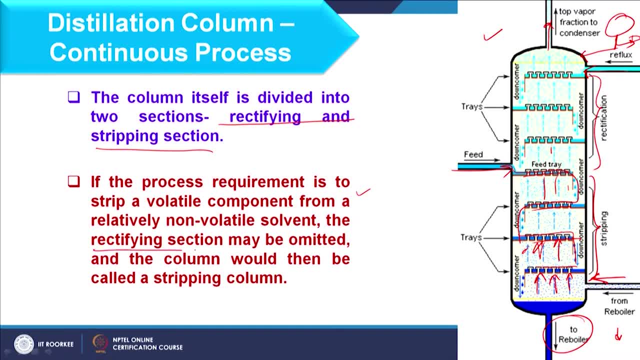 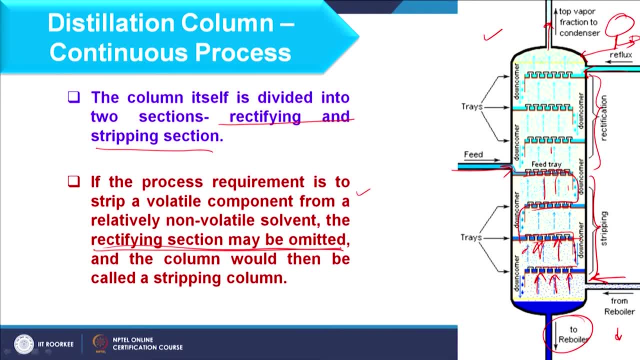 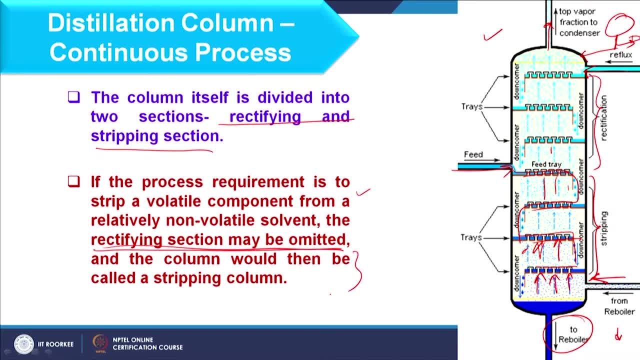 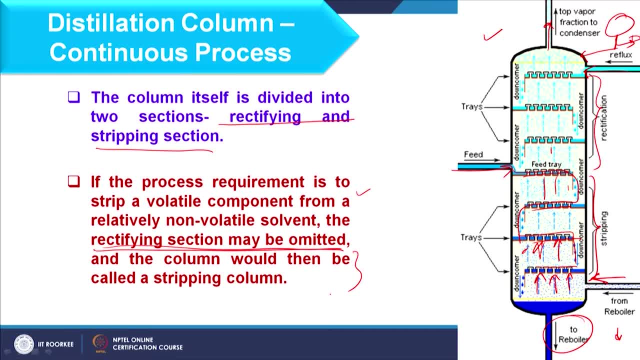 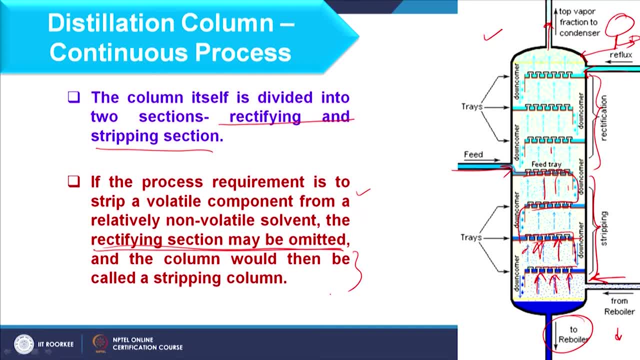 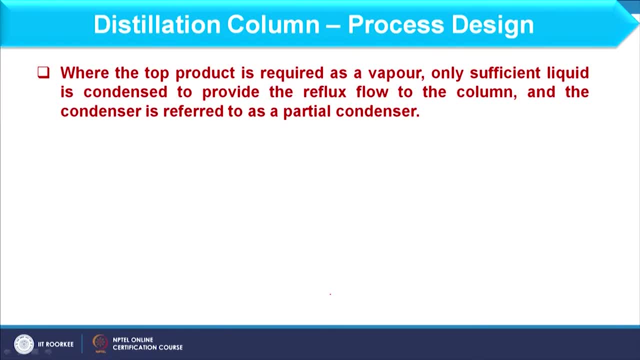 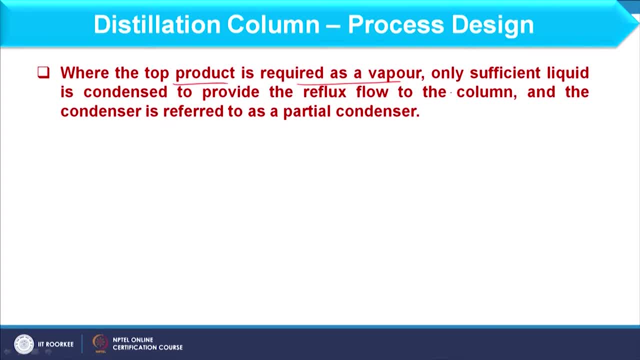 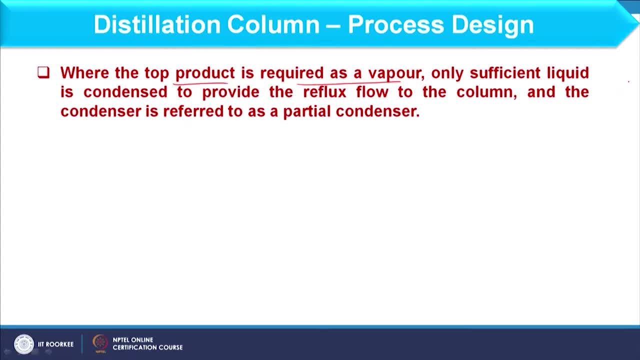 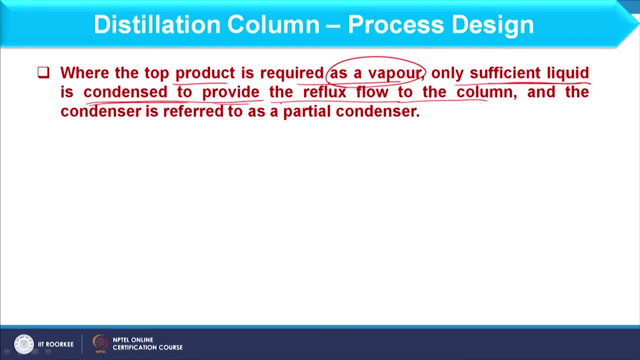 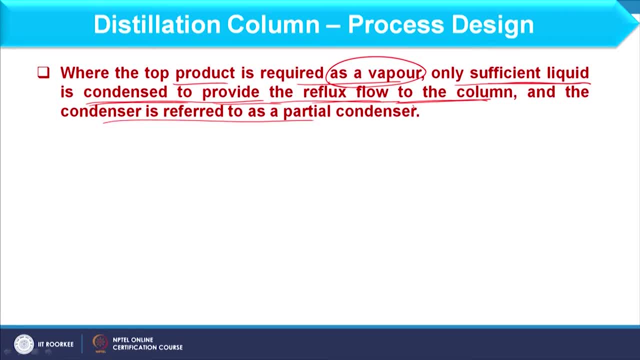 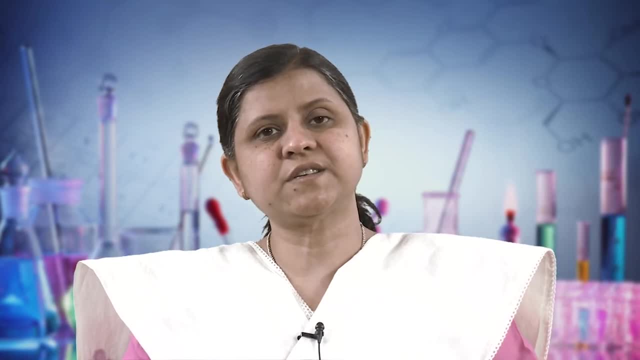 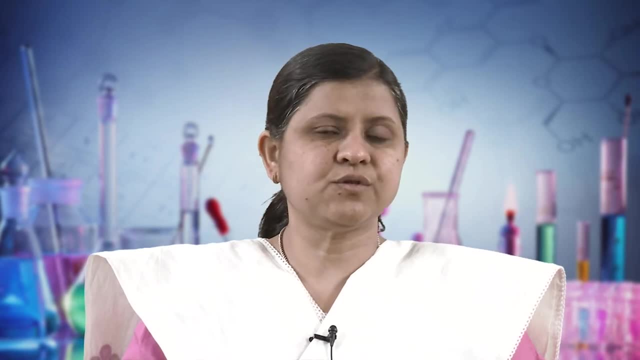 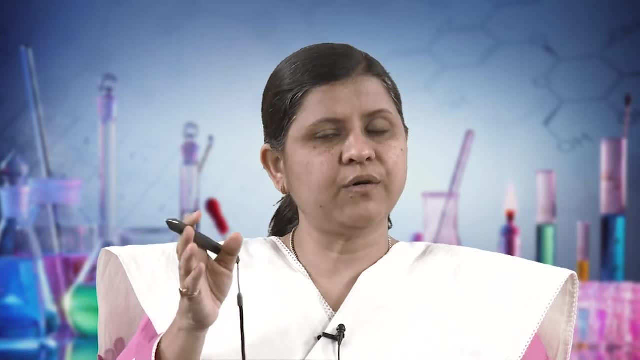 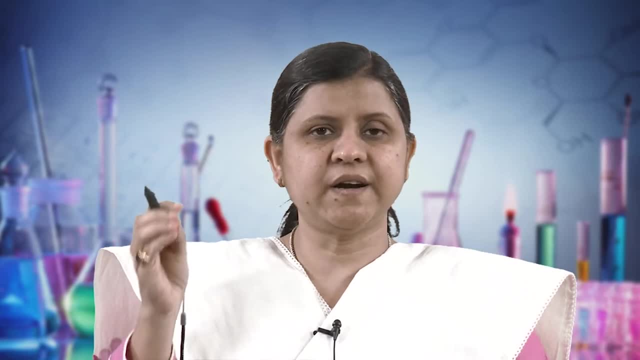 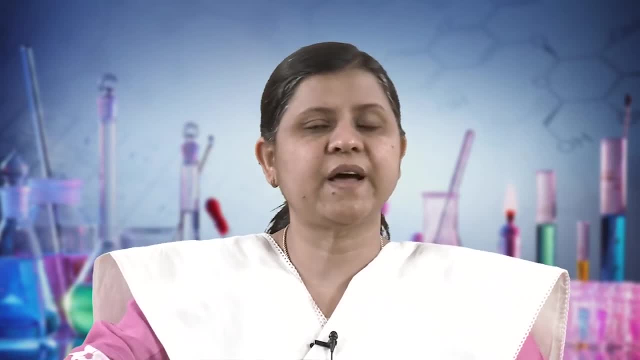 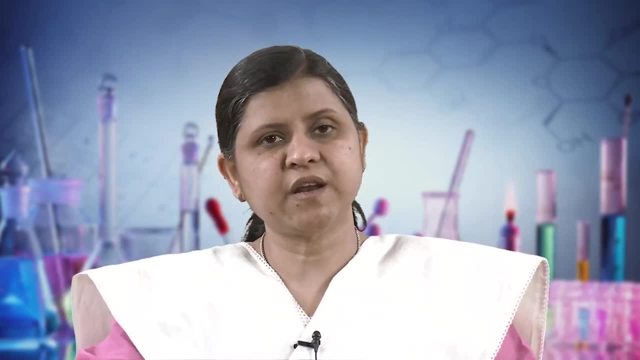 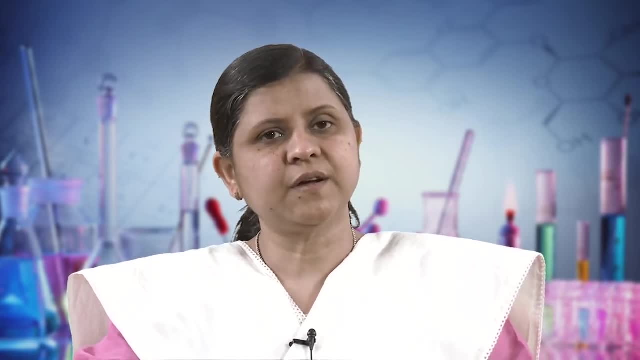 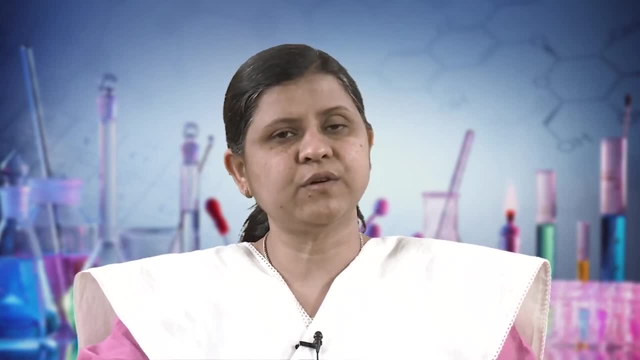 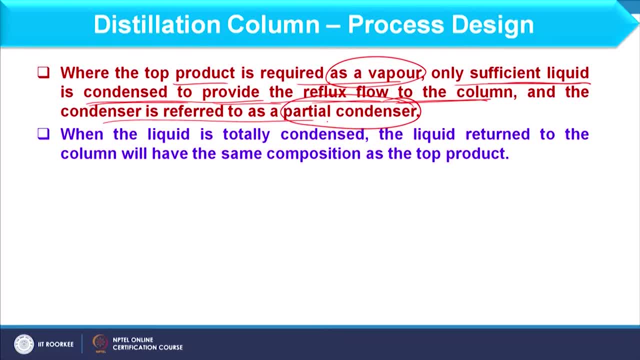 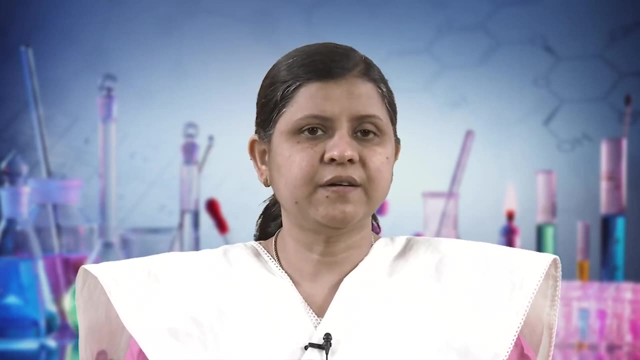 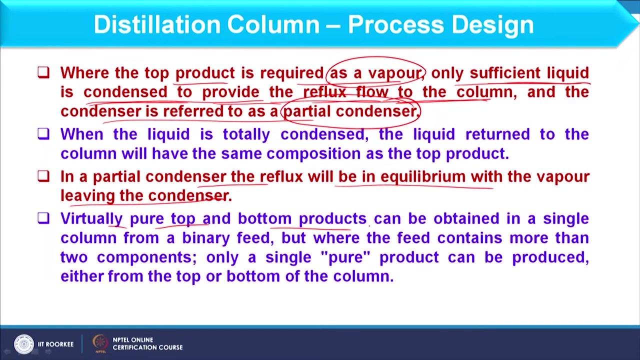 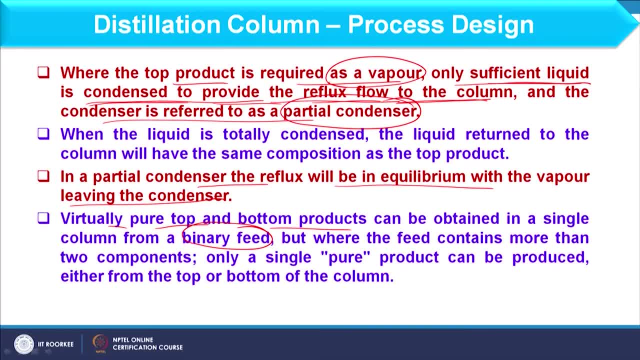 am considering binary feed. okay, But if I am having more component than 2 in the feed, only a single pure product can be obtained either from the top or bottom of the column, or usually have mixture at the top as well as bottom, okay, So this condition we call. 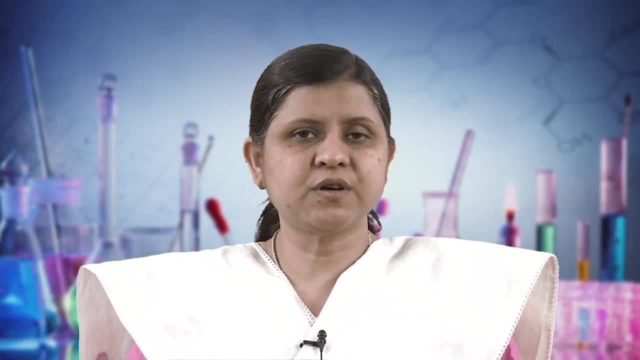 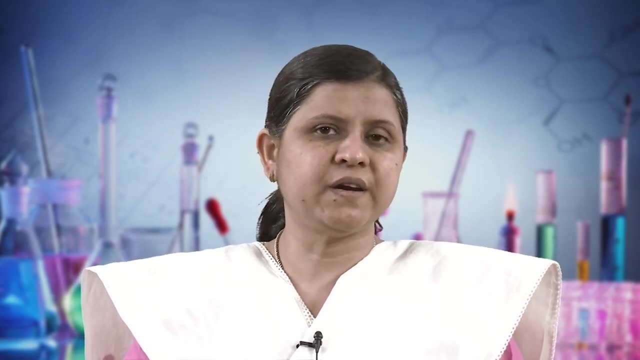 as multi-component system, and we will focus on the design of multi-component system in this course also. right, As you know, that reflux is required to maintain sufficient liquid in the distillation column, but what reflux ratio we should consider For that? so this point we have already discussed. 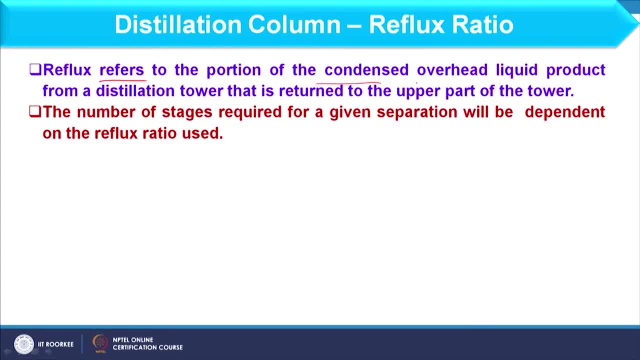 that reflux refers to the portion of the condensed overhead liquid product which is coming to the distillation column. So this is the point where reflux is required to maintain sufficient liquid in the distillation column. but what reflux ratio we should consider For that? 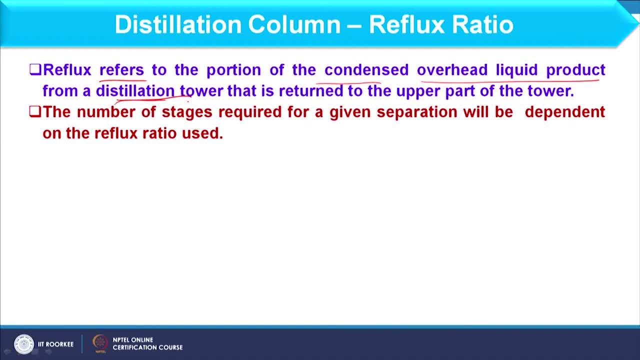 so this point we have already discussed that reflux refers to the portion of the condensed overhead liquid product which is coming to the distillation column and it is basically returning at upper part of the column. okay, And the number of stages required for the given separation will depend on the reflux. 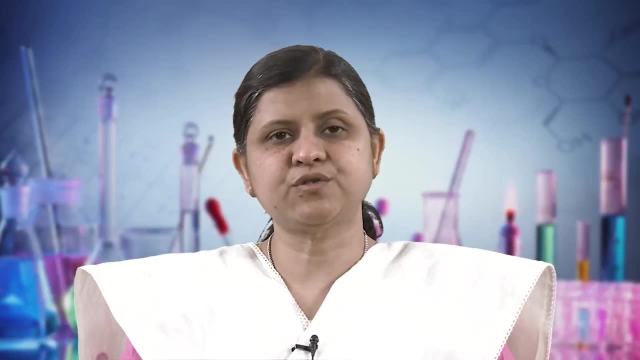 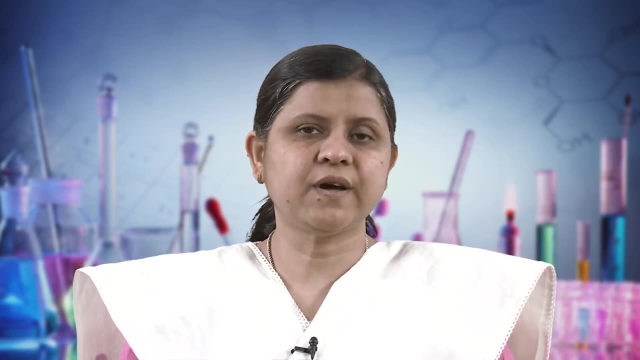 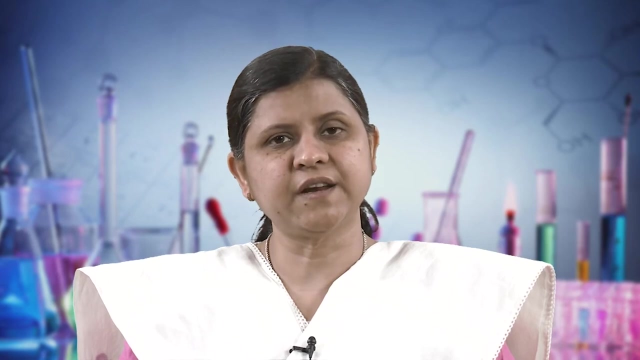 ratio. okay, As we have variation in reflux ratio, we can consider different number of stages in plate column. okay, So that you also have read with the binary system. when we consider that you also have read with the binary system, which we are going to cover in this lecture, where you 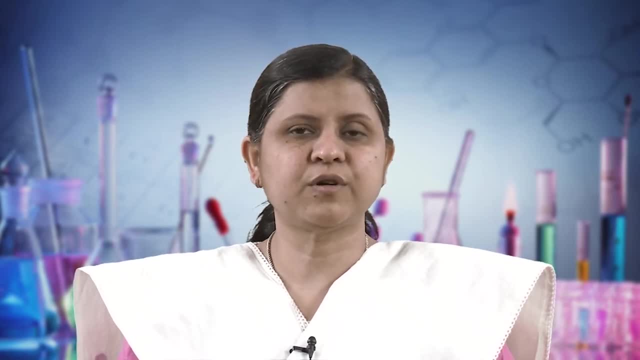 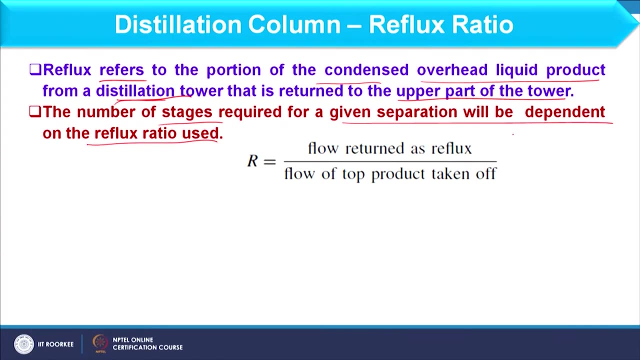 can find that, based on reflux ratio, only number of stages can be decided in McCapthley method, right? I hope you remember that method. So as far as reflux ratio is concerned, that is the flow which is returned as the reflux divided by top of the product taken off. okay, So it is basically L by D if we need to represent. 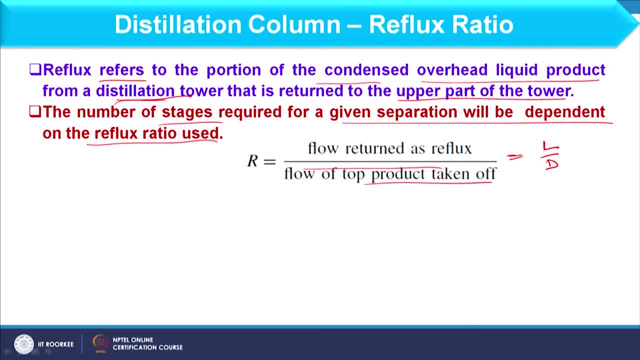 that mathematically. so that is L, which is returning back to the column, and D is the total distillate. okay, So inside the tower, downflowing reflux liquid provides cooling and partial condensation of the upflowing vapour and thereby increasing the efficiency. 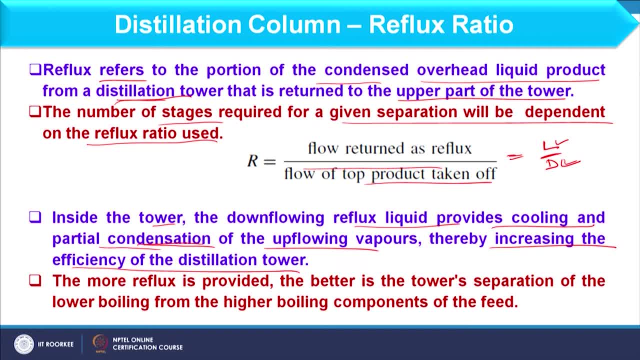 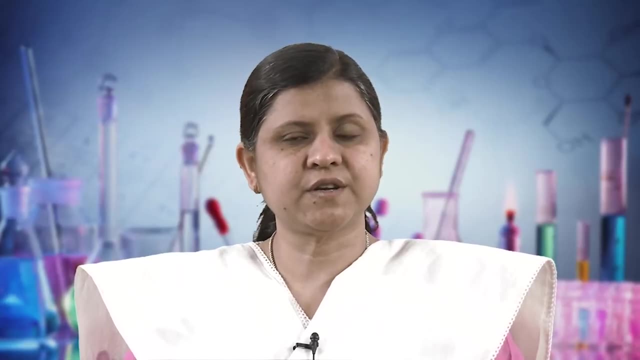 of the distillation tower. okay, So when we provide more reflux, better is the tower's separation of low boiling from the high boiling components of the feed. okay, So in this way, we consider the reflux ratio as important parameter. and let us see how to find out the reflux ratio and what are. 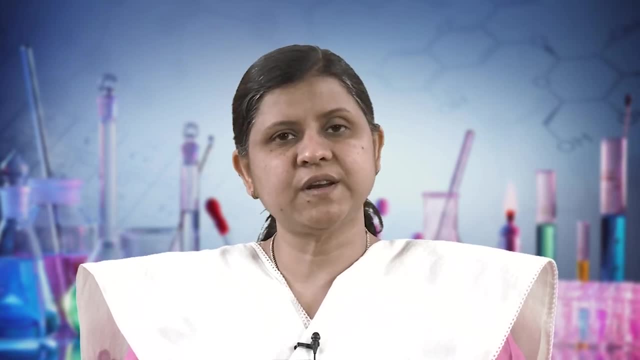 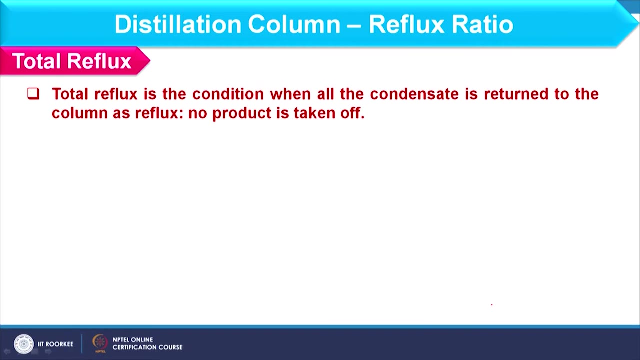 the different reflux ratio available. The first one is the total reflux. okay, So when I am considering the total reflux 1, So this all condensate is returning back to the column and in that case we are not considering any product which is exiting the distillation column from top. okay, So distillate will. 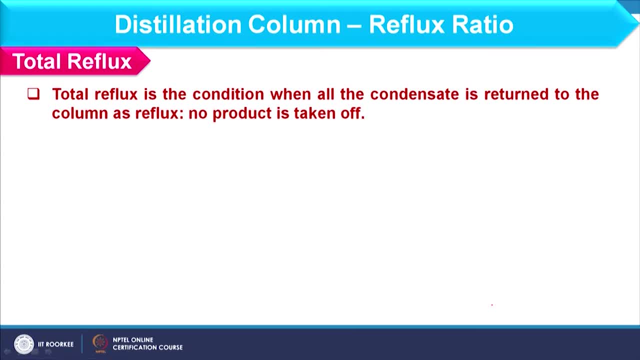 be 0,, so R value should be infinite. So in that case distillate will be 0,. so total vapour which is exiting, it is converted into condensate. okay, and that is returning back to the column 2. Now, if this is the case that we consider as total reflux, in this case number of stages- 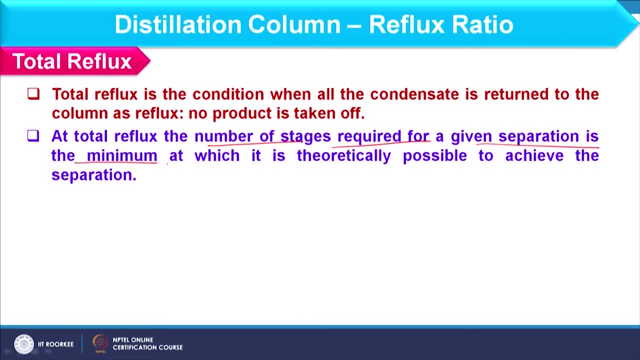 required for the given separation is minimum at which it is theoretically possible to achieve the separation. okay. So total reflux gives the minimum number of plates in the distillation column okay: 3., 4., 5., 6., 7.. 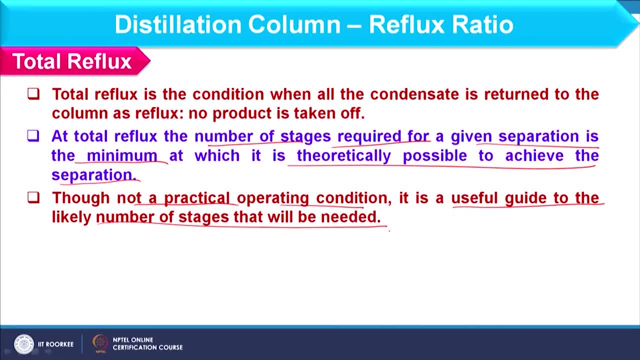 8., 9., 10., 11., 12., 13., 14., 15., 16., 17., 18., 19., 19., 20., 21., 22. 23.. 24. 25., 26., 27., 28., 29., 30., 31., 32., 33., 34., 35., 34., 35., 36., 36., 37.. 38., 39., 39., 40., 40., 40., 40., 40., 45., 40., 40., 45., 46., 46., 45., 46., 47.. 47., 48., 49., 49., 50., 50., 51., 52., 52., 53., 54., 55., 56., 57., 58., 59., 60.. 61., 62., 62., 63., 63., 64., 64., 65., 66., 67., 68., 67., 68., 69., 69., 70., 71.. 72., 72., 73., 74., 75., 76., 77., 78., 79., 80., 80., 80., 90., 92., 92., 92., 93.. 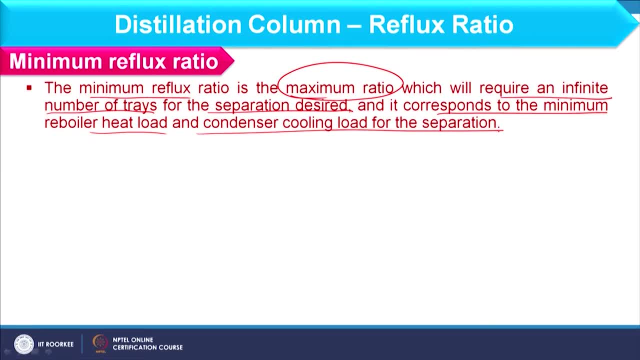 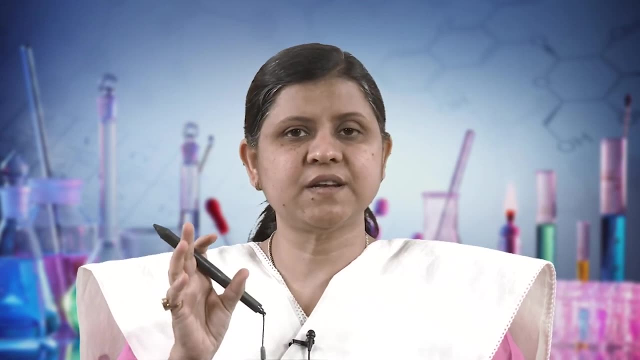 93., 94., 94., 95., 96., 96., 97., 98. 99. 100. 100. 100. 100. Okay, However, the load of the reboiler, as well as condenser is minimum, so we can consider the. 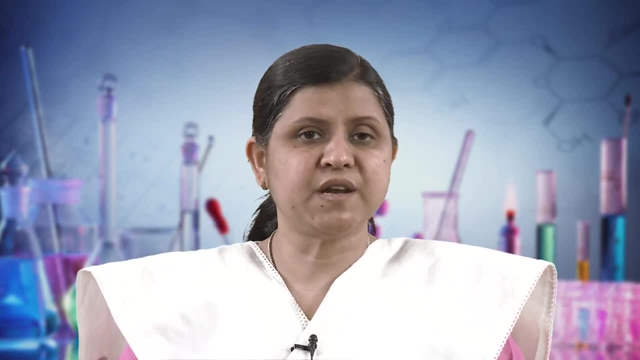 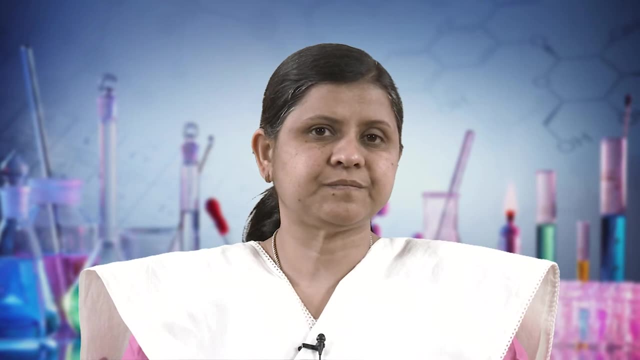 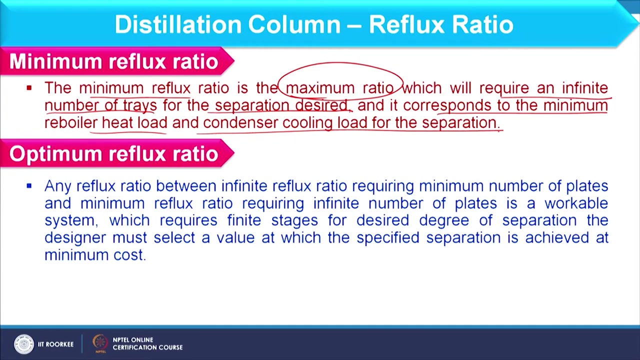 capital investment in reboiler and condenser is minimum, right. So there are two things which are moving opposite to each other and that we will consider in optimization of the reflux ratio, okay. And next we have the optimum reflux ratio, any reflux ratio between infinite reflux ratio. 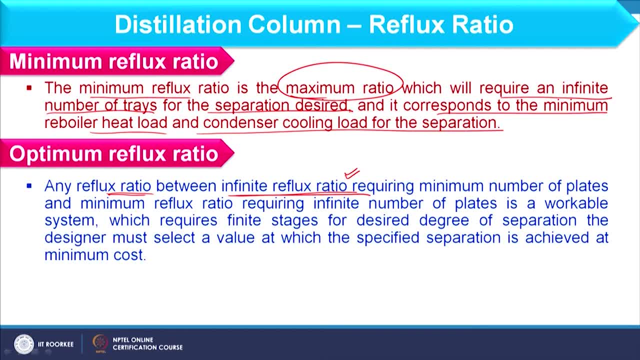 or we can consider this as the total reflux. And why I am considering this as infinite? because if r is equal to l by D, if I am not taking any product out, so D would be 0, so we can have r as infinite value. okay. 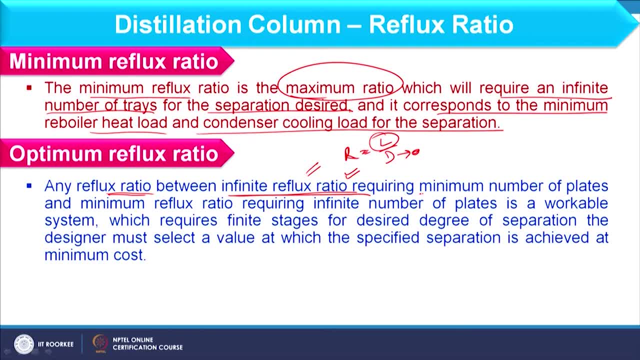 So that is also the condition with total reflux: It requires minimum number of plates, and minimum reflux ratio require infinite number of plates. Okay, okay, and we have to work between these two, fine. So we have to find the finite stages for desired degree of separation, and for that we should select the optimum reflux ratio. 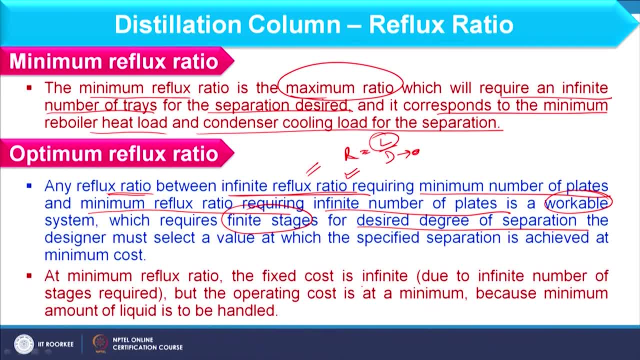 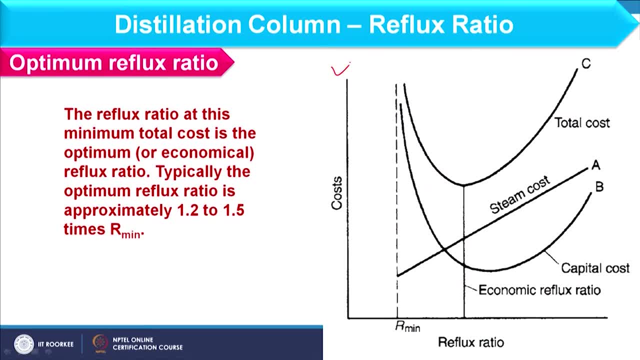 based on economic decision. okay, So let us see how to find out optimum reflux ratio. If you consider, here we have the graph between cost as well as reflux ratio. So if I have the minimum reflux ratio, we already have discussed that capital investment will be. 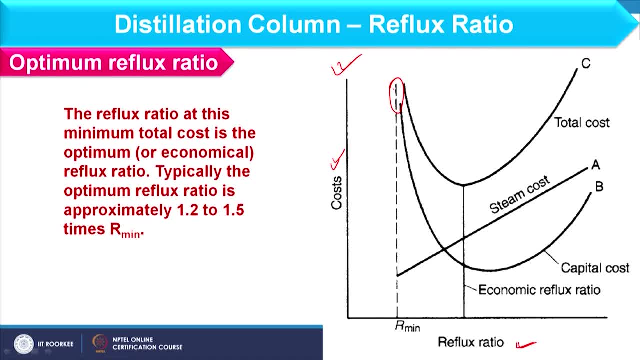 infinite, okay, but that capital investment will be in terms of minimum, but that capital investment will be in terms of number of stages, not with the cost of reboiler as well as condenser, okay, But number of stages. So number of stages will be too high that it will dominate over the cost of the reboiler. 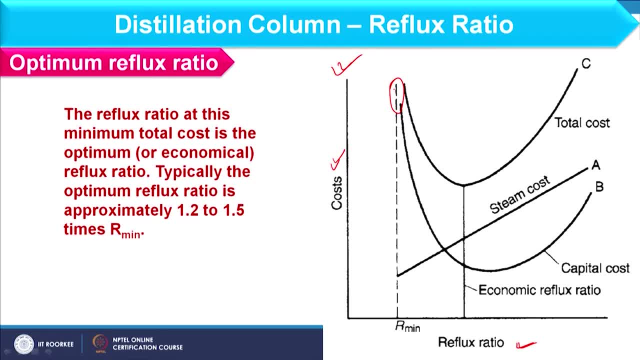 as well as condenser. okay, So when I am considering minimum reflux ratio, at that point heat duty of reboiler and condenser will be minimum, and so we can say the operating cost will be minimum, and so you can find this value where I am having the steam cost, which 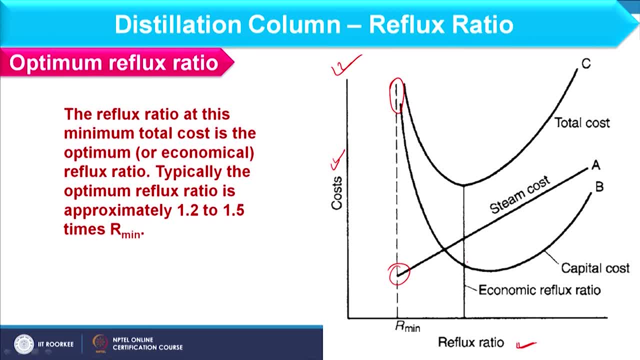 should be minimum, right, Okay. And as we move further, then the minimum reflux ratio, we can find that number of stages will keep on decreasing. okay, And when I am having total reflux ratio, number of stages will be minimum, right. In this way, somewhere we can find if this is the total reflux we can. 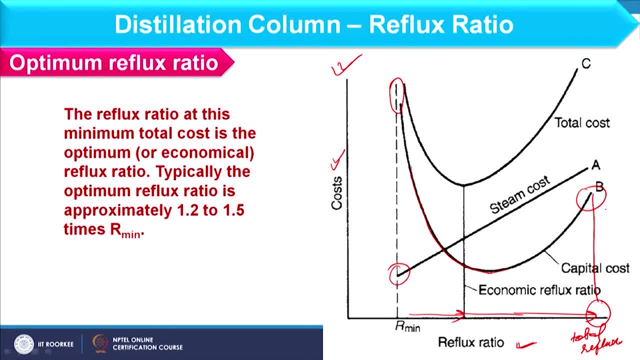 find the minimum number of stages, and capital cost due to number of stages will be least. However, at that time reboiler and condenser duty will not be less. that will be maximum. So in that case the capital cost of reboiler as well as condensate will dominate. 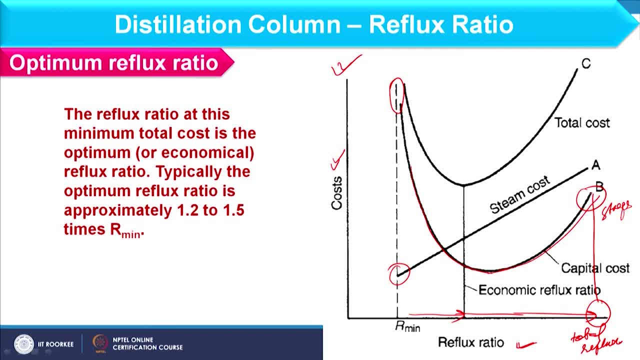 And so you can find that increment in capital investment. if this will be based on number of stages only, it should be like this. however, here it is increased, which is due to the capital investment of reboiler as well as condenser. 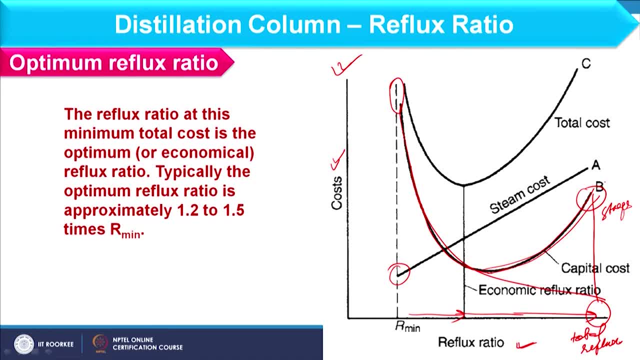 So in this way we can consider the capital investment. however, as the heat duty will increase from minimum reflux to total reflux. however, as the heat duty of reboiler and condenser increase with the total reflux, So the increment in reflux ratio from minimum reflux to total reflux, we can continuously. 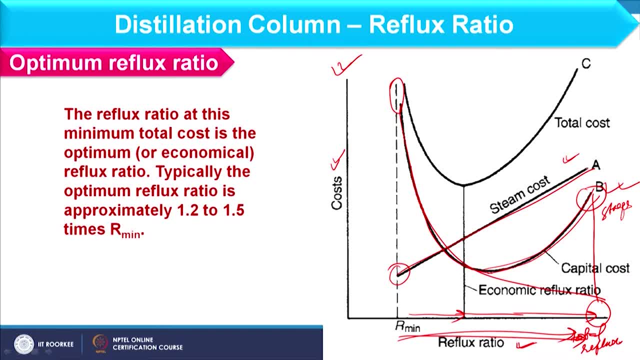 find variation or increment in the operating cost, And if we consider addition of these two we can find total annual cost, and wherever it will give the minimum value, this reflux ratio I can choose as the optimum reflux ratio, right? So usually optimum reflux ratio can be calculated in the following manner: 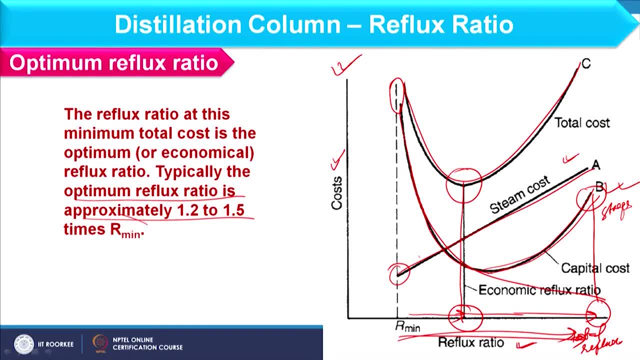 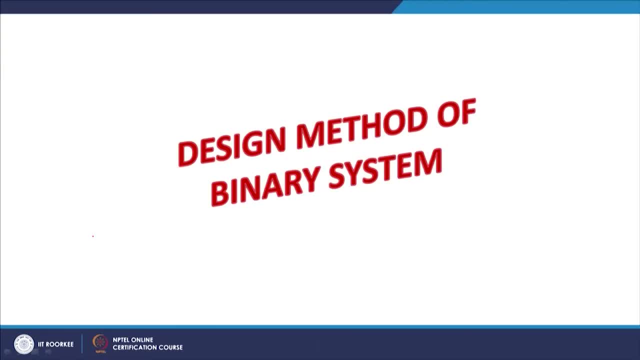 reflux ratio is approximately 1.2 to 1.5 times minimum reflux ratio. okay, So in that way we can choose the optimum reflux ratio. and now we will discuss the design of binary system. Why I am considering this? because whatever balances we consider in binary system either 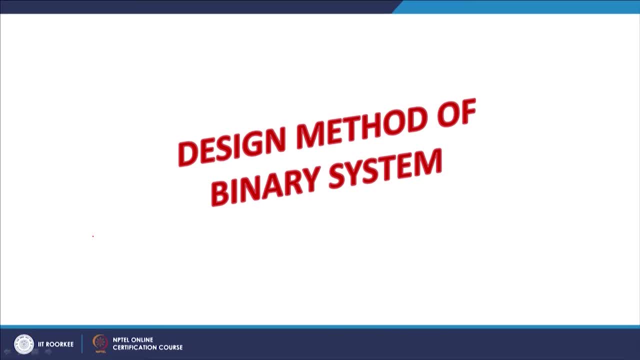 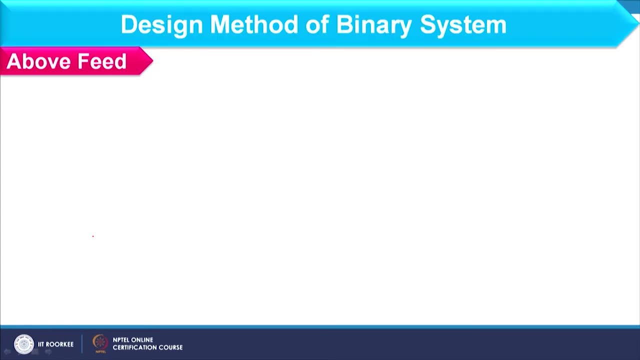 mass balance or energy balance. the same will be extrapolated to multi component system also. So here we will revise the design of binary system, assuming that you know, or assuming that you know, this already. okay, So to design the binary system, let us make the. so to start, 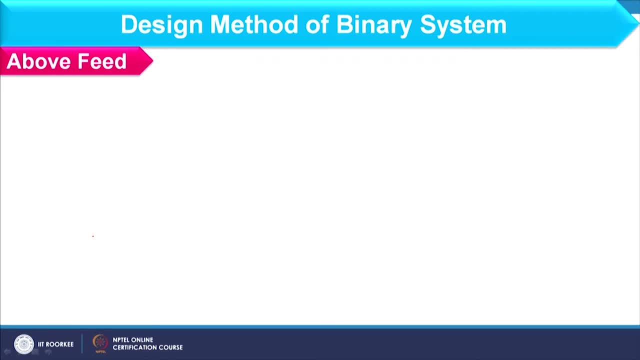 design of binary system. let us make the material as well as let us make the material and energy balance. okay, So we are considering above feed system, so here you can consider the distillate And this is basically the reflux. and if we consider material and energy balance, we usually 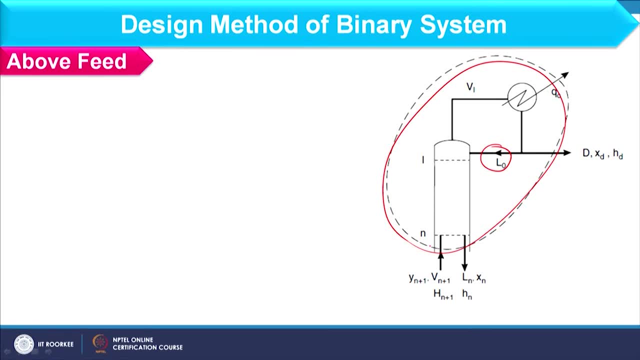 make the envelope and in this envelope, whatever stream is entering, is that Vn plus 1 that is available. that is basically the vapor stream which is exiting: n plus 1th tray, right, It has composition as Yn plus 1.. And total energy which is and total enthalpy which is available in this is capital H n. 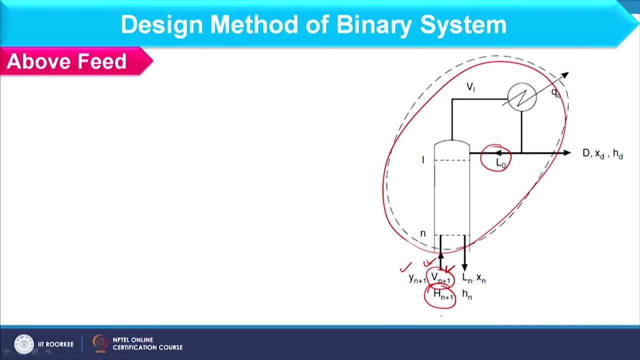 plus 1,. okay, So that you understand that for vapor we represent the total energy or total enthalpy in the form of H. In the similar line streams which are leaving the system are Ln available at Hn, at composition, Xn right And. 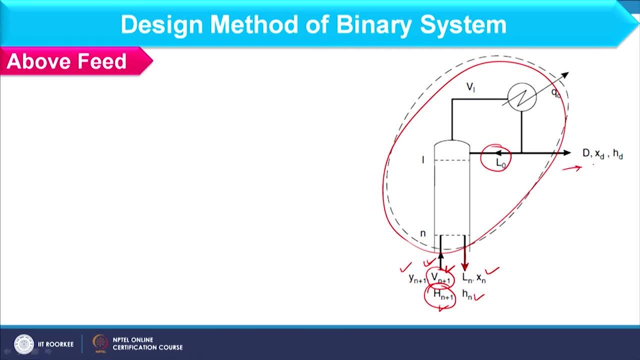 Transition, Another Stream From which is exiting. the system is distillate at xd containing enthalpy hd. So making the material balance we can simply consider Vn plus 1 should be equal to Ln plus d. simple balance is there and for component balance we can consider as Vn plus 1 into. 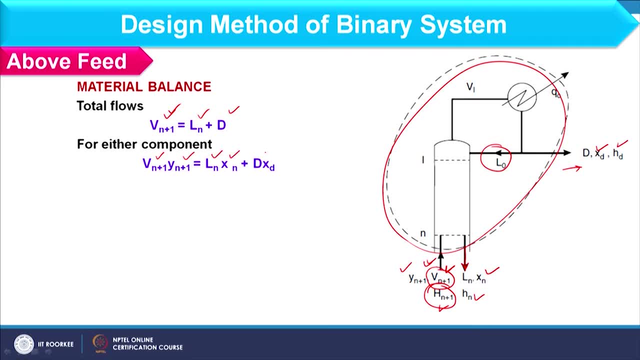 Yn plus 1, equal to Ln, into xn plus dxd. In this way we can make the component as well as mass balance. Now we can make the energy balance. total streams enthalpy because this is basically stream which is entering and that contains Hn plus 1, so this is the simple balance and 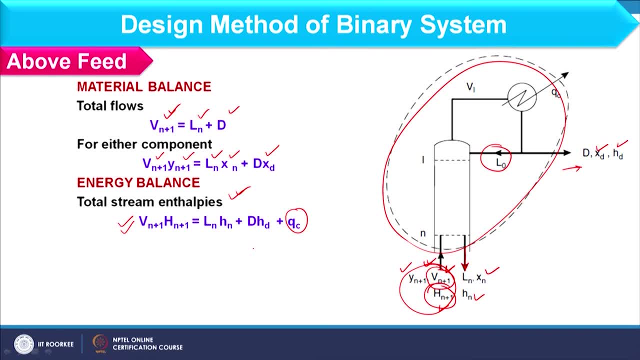 here we are considering Qc, because Qc heat which is released from the condenser, it means this amount of heat is coming to the coolant from vapour stream, right, So we consider that this heat is exiting the system, okay, So here you see. Qc is basically heat removed from the condenser. that we have already discussed. 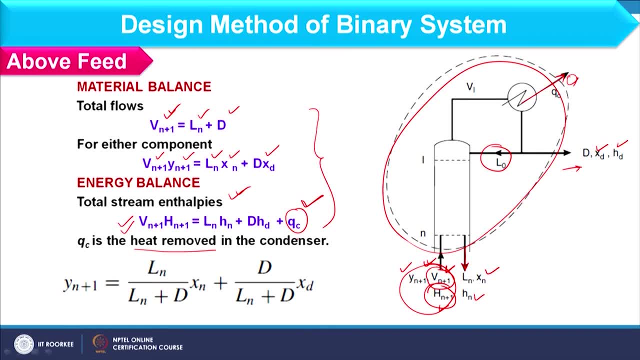 Now arranging these equations, we can find the final equation as Yn plus 1 equal to Ln by Ln plus d xn. Okay, So in the similar line I can write the enthalpy balance also. okay, replacing this Vn plus 1 with this. so we can find this expression okay. 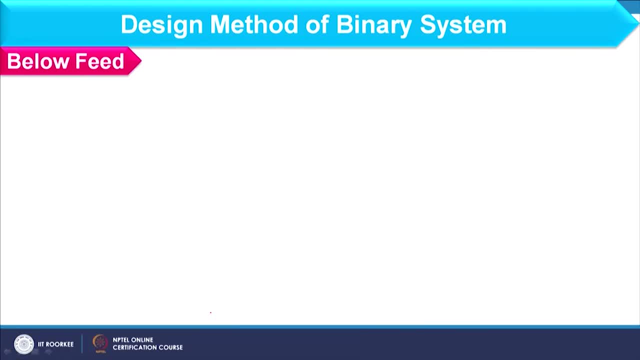 So these are basically the equations for above feed condition. Now, similarly, we can find the balance at below feed and here we can make the balance and making the envelope like this: Okay, simple balance will give. so I am not going into detail of derivation of the equation. 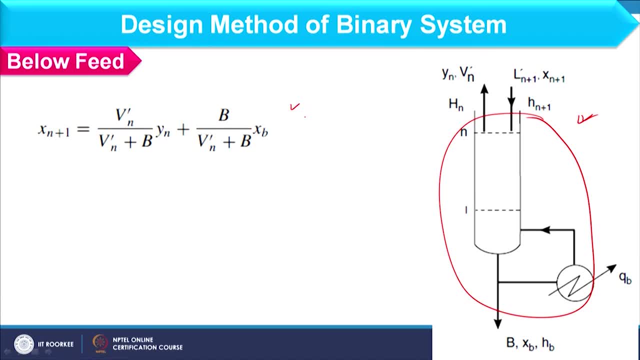 we can simply have the equation as xn plus 1, which will be equal to V dash n by V dash n plus b into Yn, and then plus, and we can have b by V dash n plus b into xb. So you can see, here we are representing the vapour flow rates as well as liquid flow rates, with. 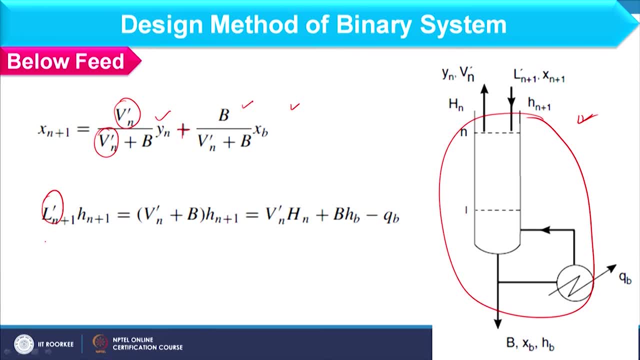 prime. okay, So that is the basic representation of variables in above feed and below feed. columns right. So below feed we usually consider prime, above feed we consider without prime. So in subsequent lectures also if this nomenclature is used, you should understand which part I 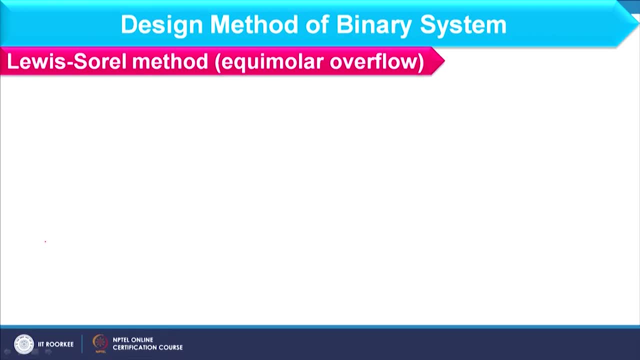 am focusing on: okay. Okay, Now further, we can have some assumptions and based on that we will design the binary system. The assumption says: as the assumption is like, whatever molar flow rate we are considering, either for liquid and vapour, so these molar flow rate will be constant in each tray. okay, 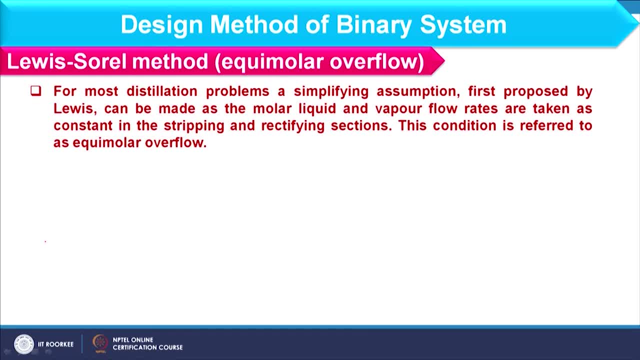 So throughout the distillation column, these vapour flow rates, as well as liquid flow rates, will be constant, Like if I am considering Ln or Vn- okay, so that should be LnV throughout the distillation column, and that assumption is basically given by Lewis. 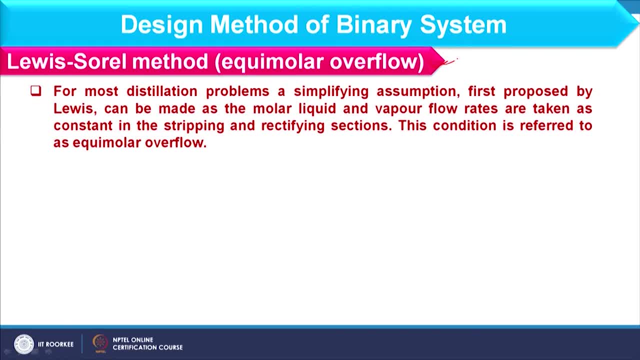 So complete method we call as the Lewis-Sorel method, and here the assumption is like molar liquid and vapour flow rates are taken as constant in stripping section and rectifying section. Okay, Okay, So this is what we call as equimolar overflow. 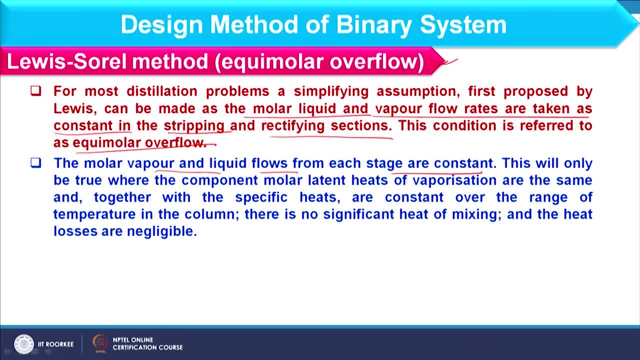 So the molar vapour and liquid flows from each tray are constant. that is the assumption only, and this will be true where component molar latent heat of vaporization are same and, together with the specific heats, are constant over the range of temperature in the column. 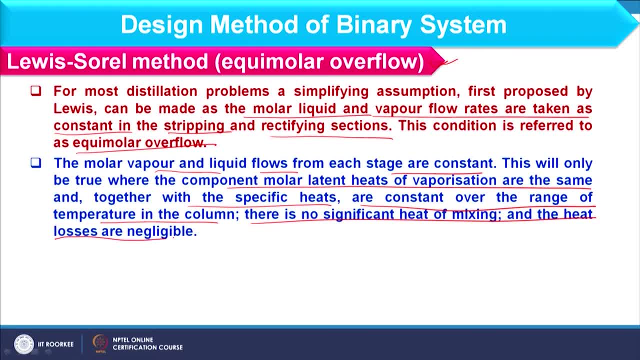 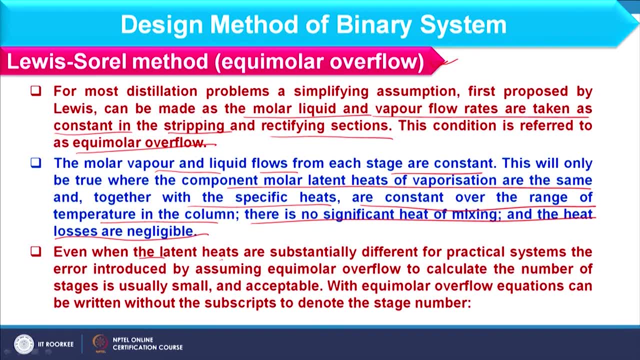 and there is no significant heat of mixing, and heat losses are also negligible. Okay, Further, even when latent heats are substantially different from the practical system, the error introduced by assuming equimolar overflow to calculate number of stages is usually small, and that can be acceptable also. 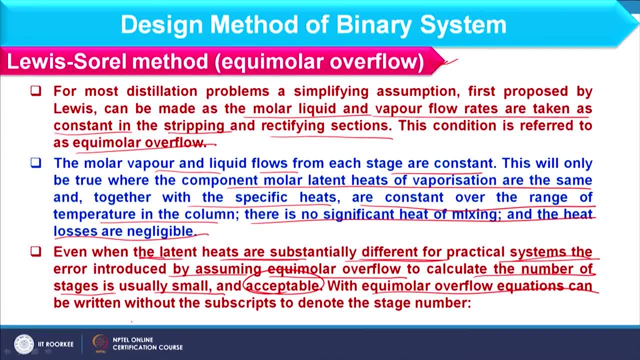 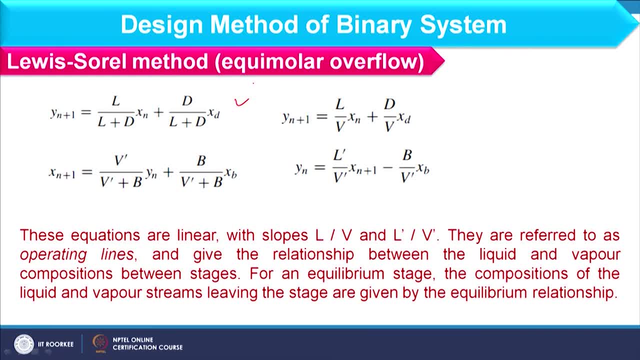 Thank you. Okay, So when I am assuming this, we can represent the equations like: Yn plus 1 should be equal to L by L plus d into x, n, and additionally we further consider d by L plus d, x, d. Okay. 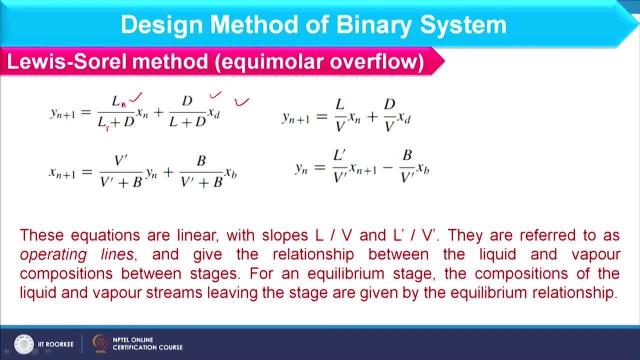 So you can see we are not considering n over here like this: Okay, not be considered, because equimolar overflow we have assumed and when we resolve this equation, we can obtain equation like this. and when we consider this equation, we can find revised equation as like this: simply rearranging and considering the balances. 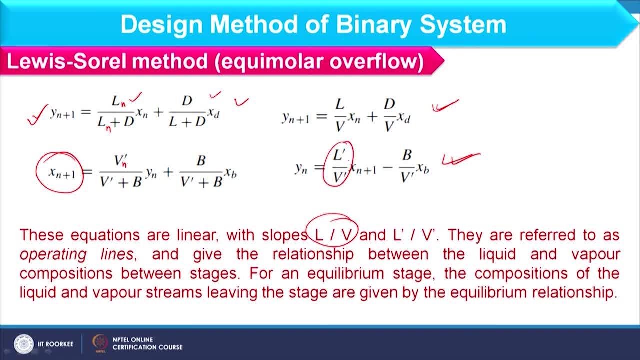 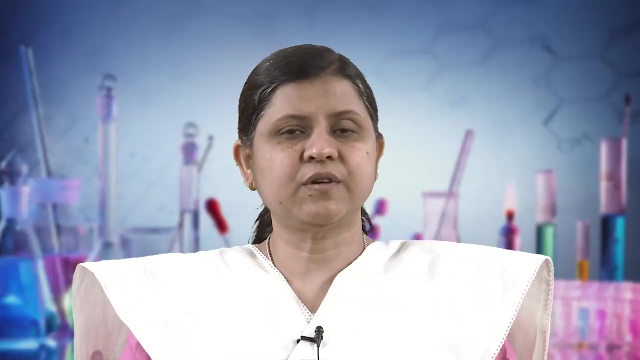 So in this equation L by V and L dash by V, dash are basically the slopes and they are referred as the operating lines and give relationship between the liquid and give relationship between liquid and the vapour composition, between stages. for an equilibrium stage, the composition of liquid and vapour streams leaving the stage are given by equilibrium relationship. okay, 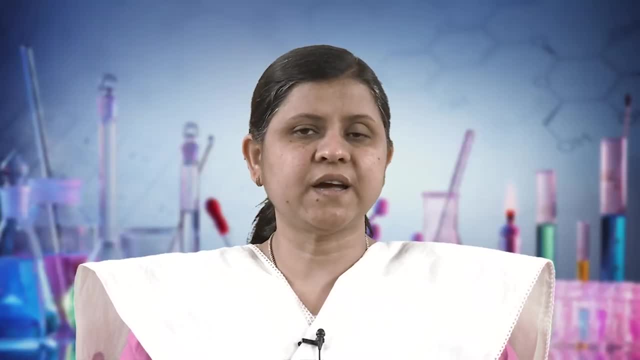 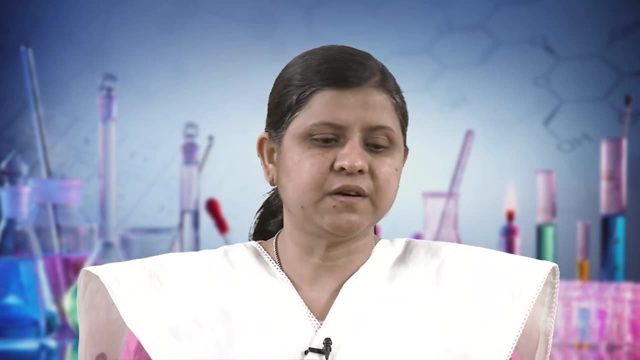 So these are some points which we have to discuss to design the binary system. and here we are having. So let us see the steps to be followed in this method. So initially we have to plot the vapour-liquid equilibrium curve from the data available. 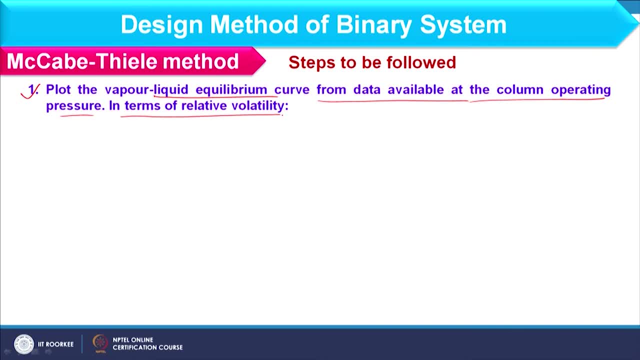 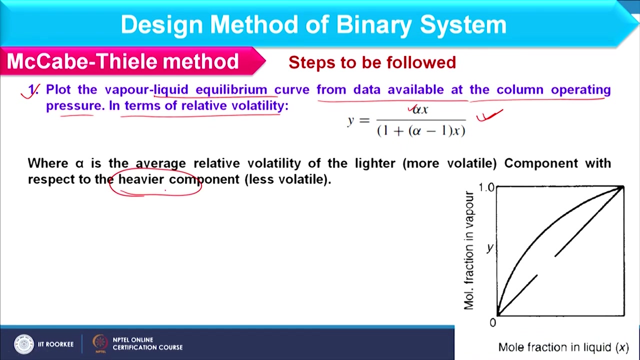 at the column operating pressure and in terms of relative volatility, and we can consider that equilibrium curve with this equation right. So where alpha is basically the relative volatility of lighter component and that equilibrium curve is the relation we consider with respect to heavy component, okay, 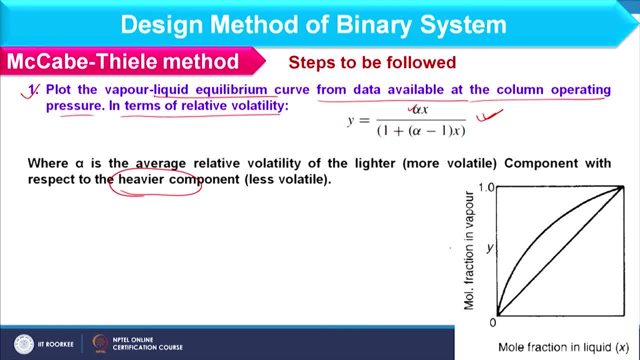 So you can see, here I am having mole fraction in vapour that is y as well as x on x-axis and, if you see, this is basically the equilibrium line and plotting these and joining these two point will give this line, okay. So volatility of A: it is defined as the ratio of partial pressure of A to the mole fraction. 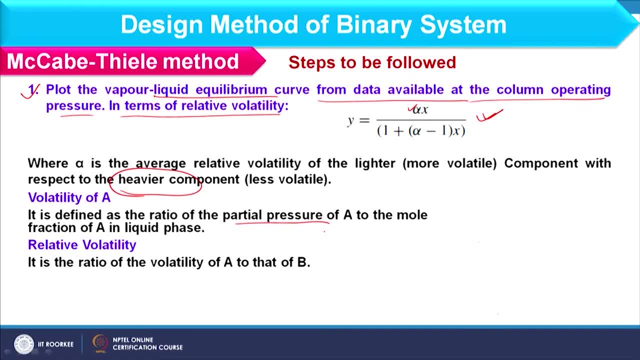 of A in the liquid phase and relative volatility, it is the ratio of volatility of A to that of B. okay, So you can consider these equations: when I am having alpha and when it is equal to 0,. when I am having alpha equal to 1, it means no separation occurs, and when alpha is there. 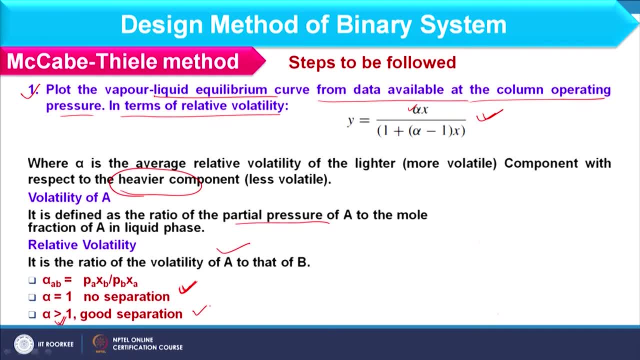 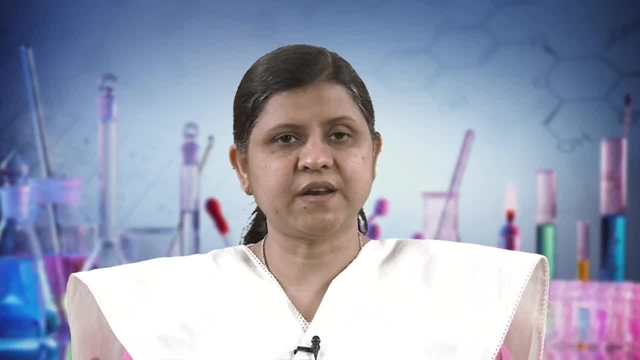 which is greater than 1. we consider that as good separation condition. so these are some nomenclature Which we consider in McCabe-Thiele method or distillation column designing. okay, And further. second step is to make the material balance over the column, to determine top and. 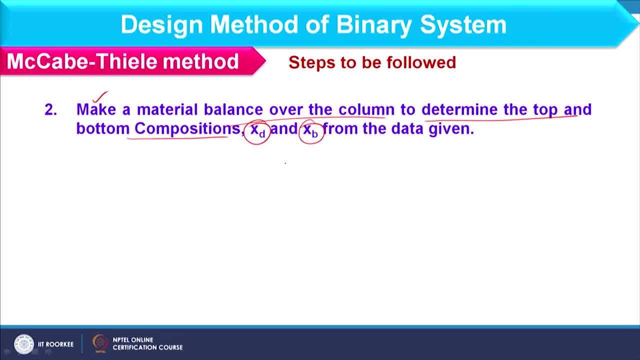 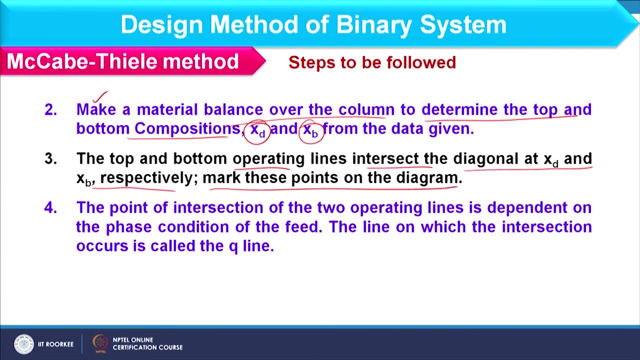 bottom composition, that is xd as well as xd. from the given data, The top and bottom operating line intersect the diagonal at xd and xb respectively and we have to mark these points on the diagram. okay, We will see that You can see all these points in the diagram also in the next slide. 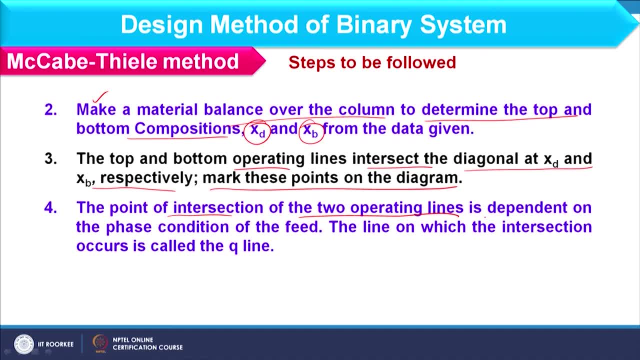 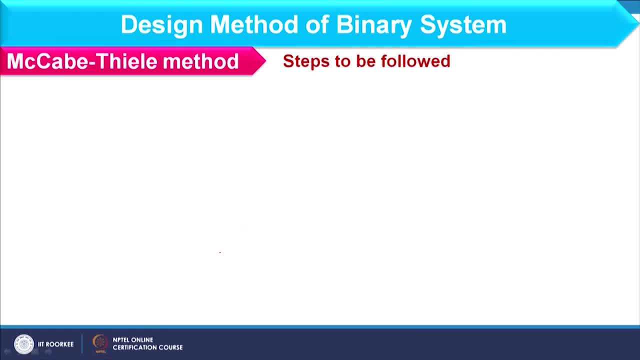 The point of intersection of two operating lines is dependent on the phase condition of the feed, and so we consider the q line okay, And this q line can be considered as q should be equal to heat to vaporize 1 mole of feed divided by molar latent heat. 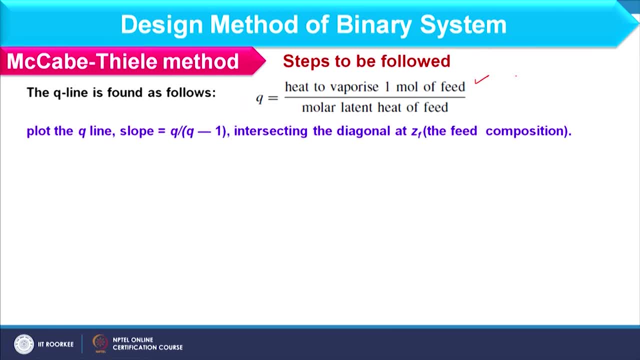 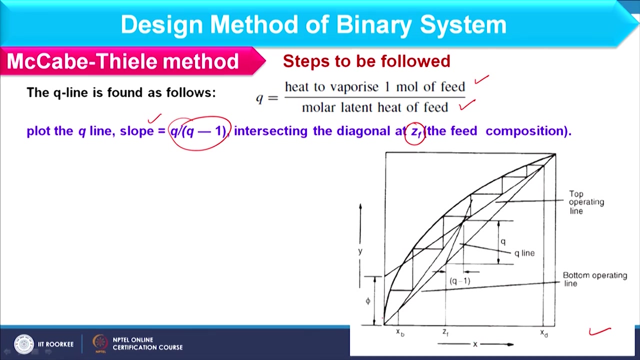 Okay, So we can plot the q line with the slope which is equal to q by q minus 1 and intersecting the diagonal at zf, which is basically the feed composition. So if you consider this graph, here I am having the same curve, that is, the equilibrium curve. 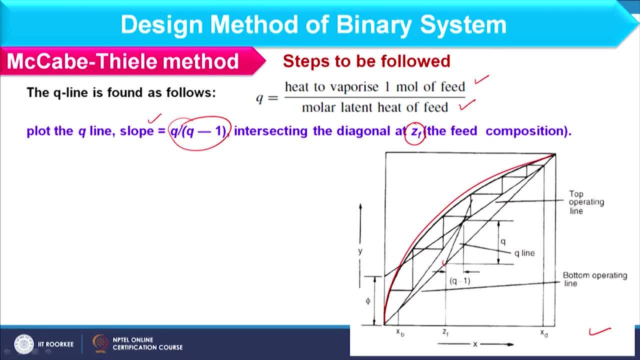 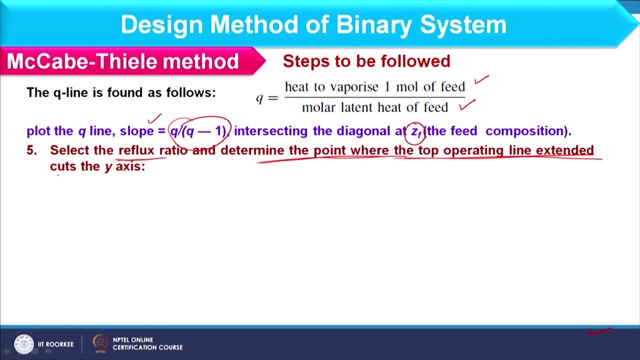 okay, like this. Okay, And here I am having the feed condition And from this I can draw the q line. okay, So that is basically the q line and then select the reflux ratio and determine the point where top operating line extended which cuts the y-axis right.